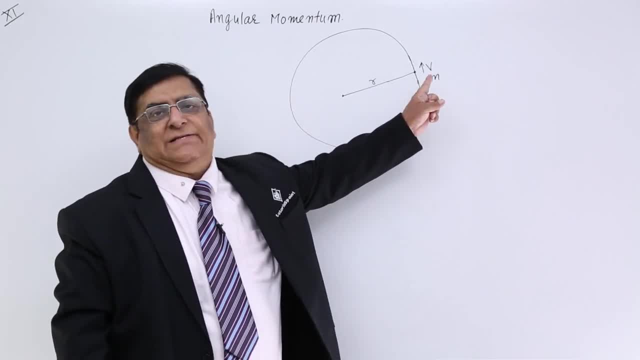 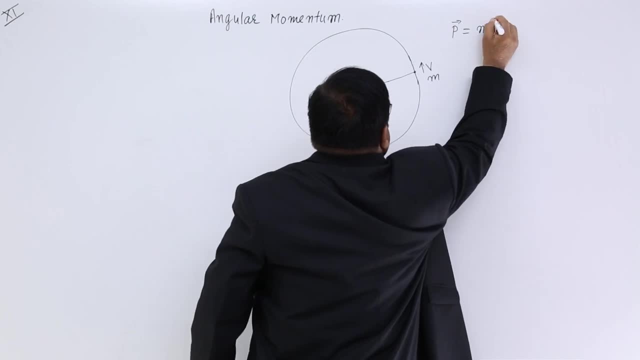 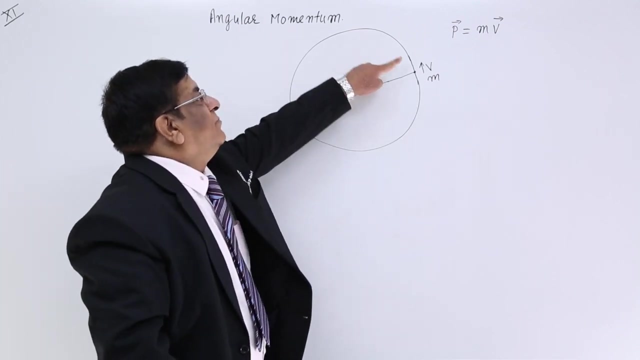 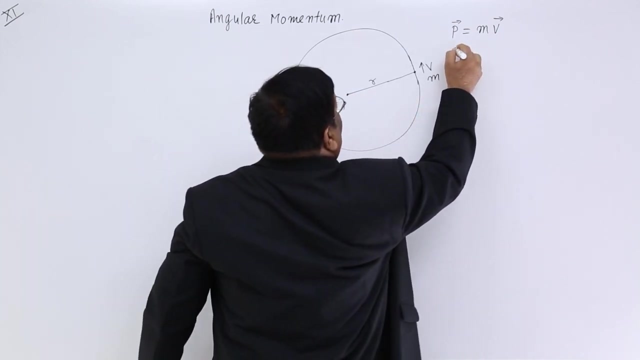 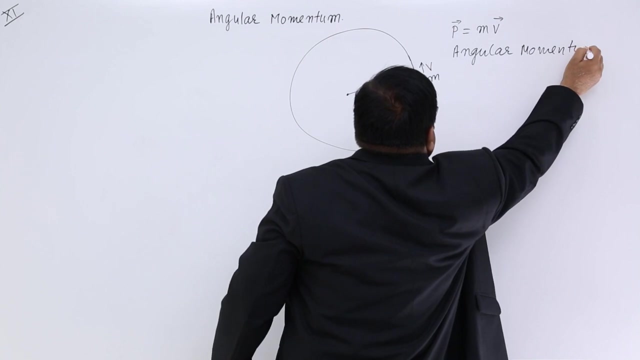 Now there is a physical quantity known as linear momentum. Normally we mention linear momentum. m into v, Mass, into linear velocity is linear momentum. Now this momentum has effect in this rotational motion and that effect is known as angular momentum. What is the angular momentum quantity? 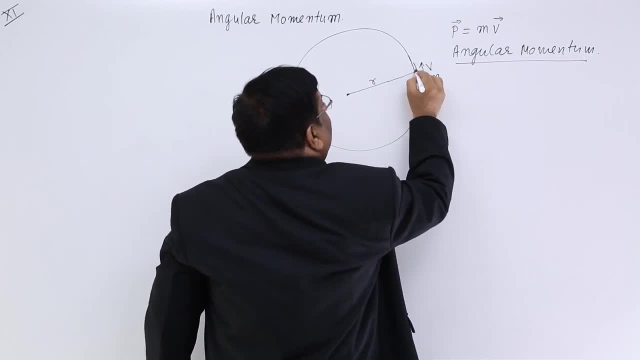 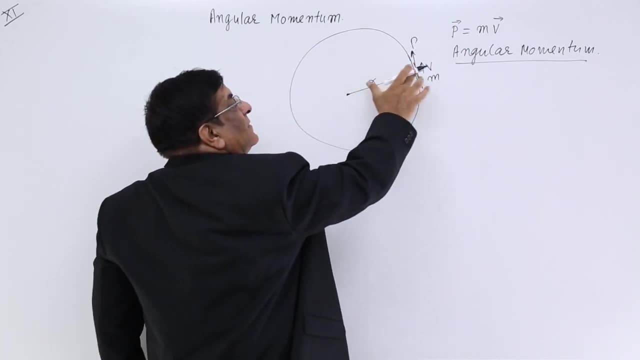 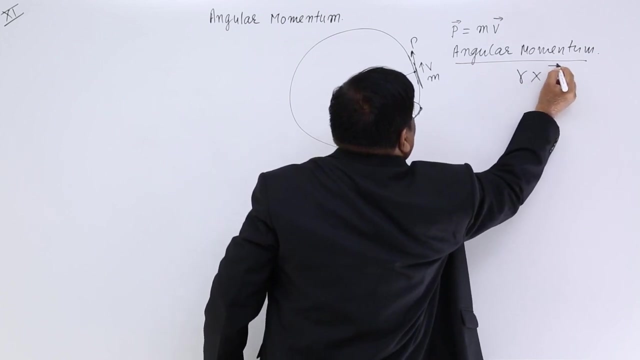 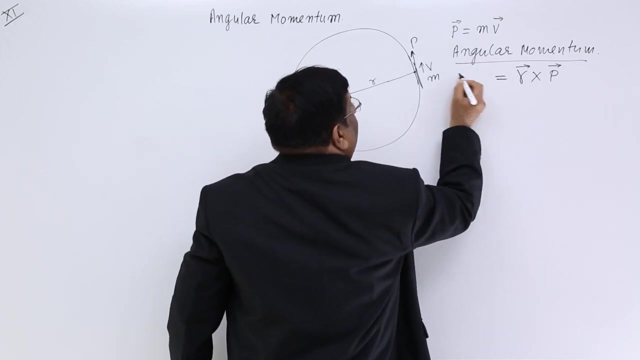 When we multiply linear momentum p here linear momentum p, with this arm of rotation, then it affects increase. So r cross p becomes a quantity in angular motion, in circular motion, which we will call angular momentum, and we give it a symbol m. 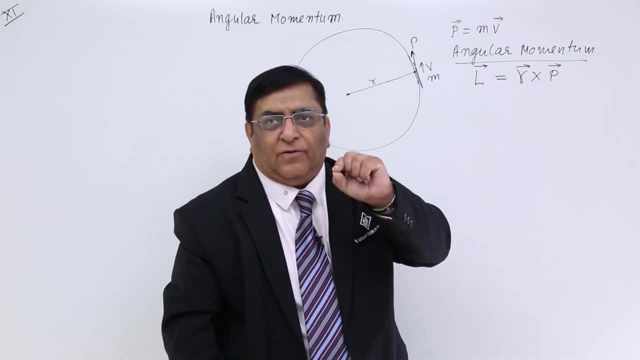 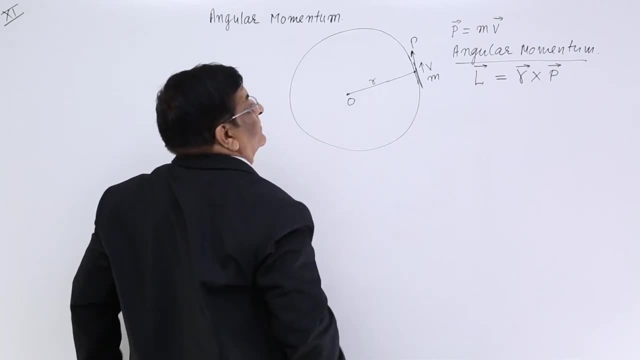 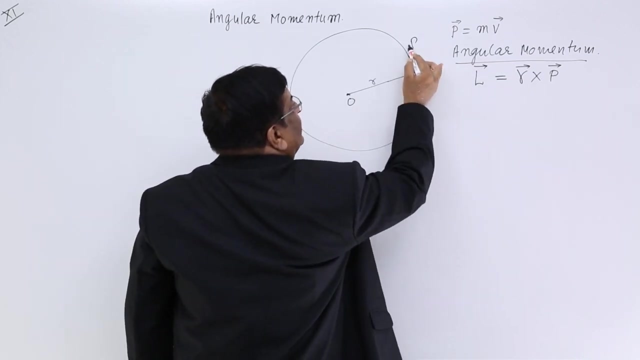 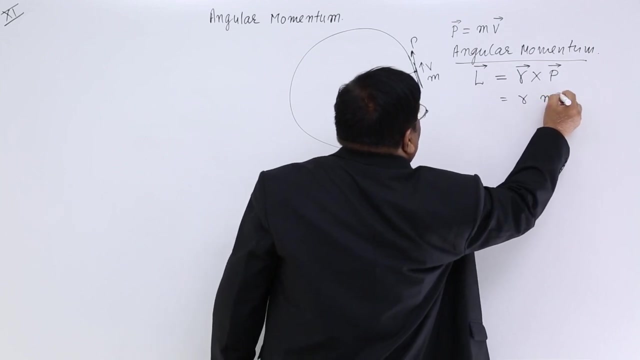 So angular momentum is effect of a body which is rotating around a point. So this is r cross p, where r is the arm of rotation and p is the linear momentum at this particular point. Or we can say this is r into mv. 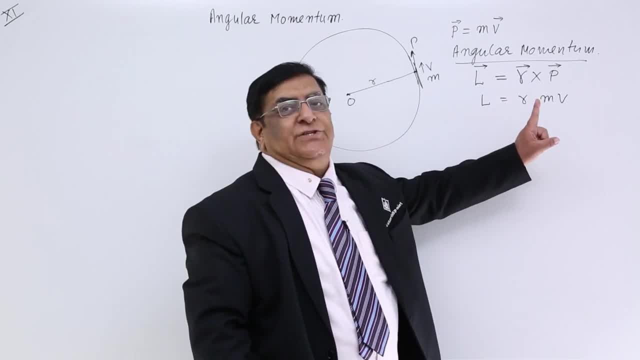 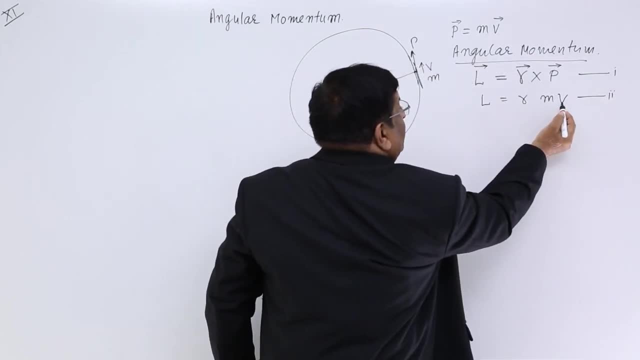 Now we have other conversions. also, If v- linear velocity- is m, then we have plus or minus mv. So this is r cross p. So this is r cross p, Where r is the arm of rotation and p is the linear momentum at this particular point. 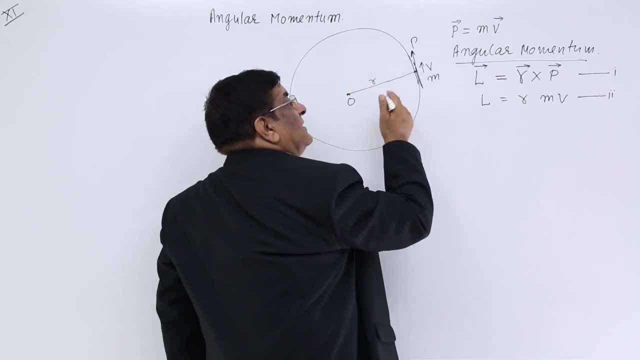 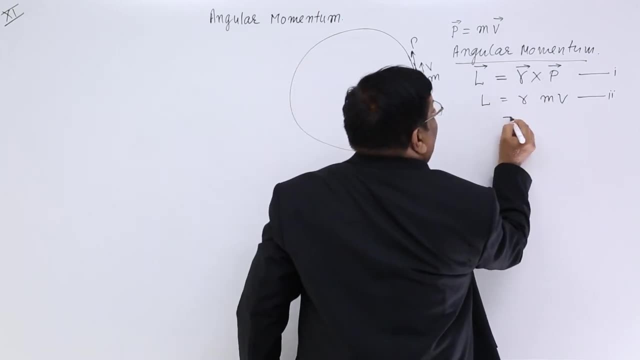 Or we can say: this is r into mv. Ok, is converted into angular velocity omega. We know the relation V is equal to r omega. That we put here r omega And what we get here is r omega. So that makes it m? r square into omega. This is angular velocity, angular momentum. 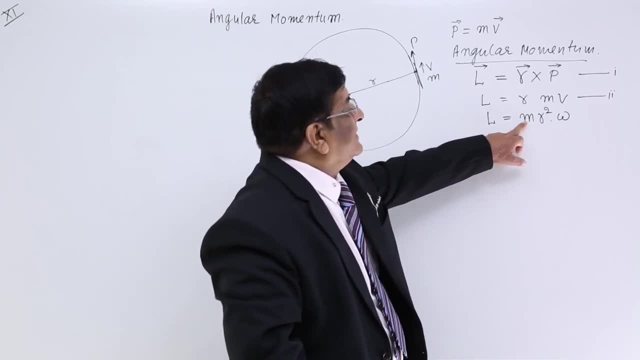 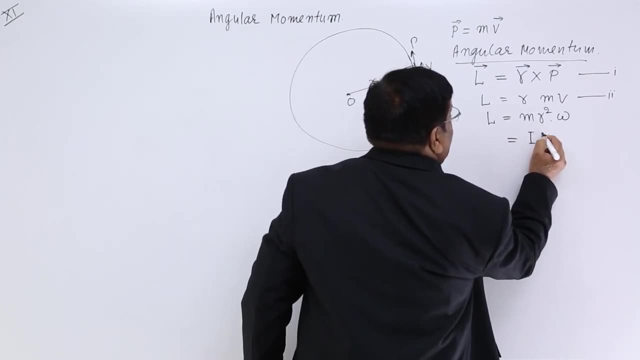 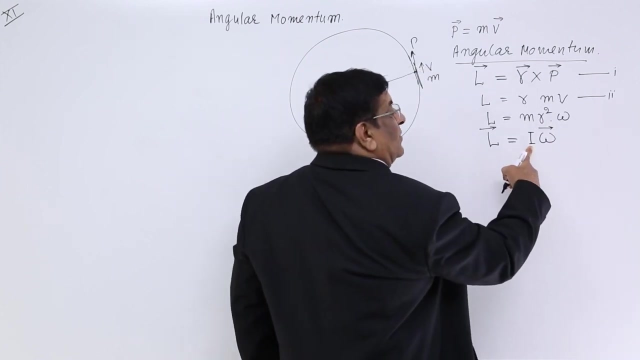 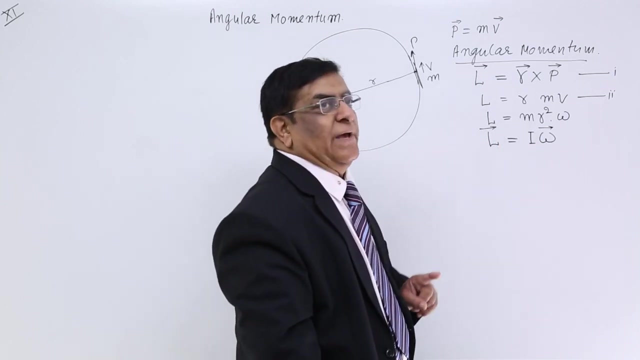 Now m r square is a known term to us. This is moment of inertia. So what we get here is i into omega. This is l. This is scalar quantity. L is equal to i into omega. Now l has got direction of omega. Omega has direction along the axis, So l is also having. 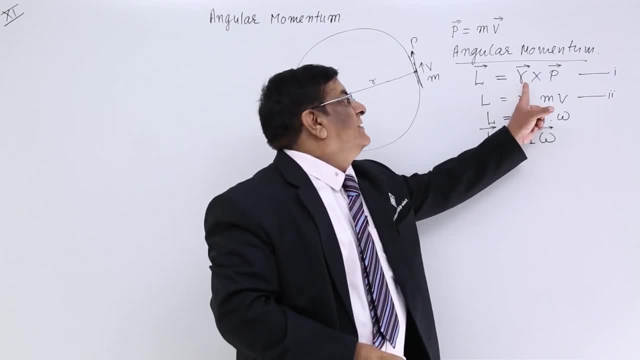 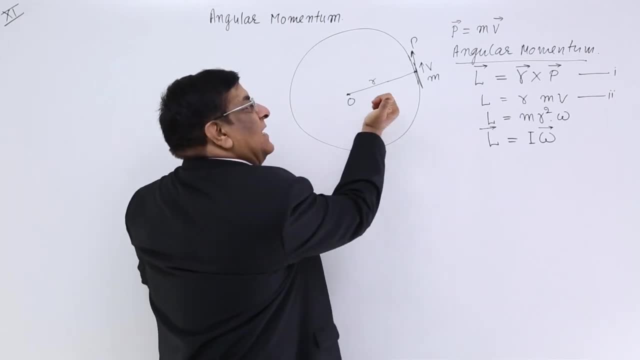 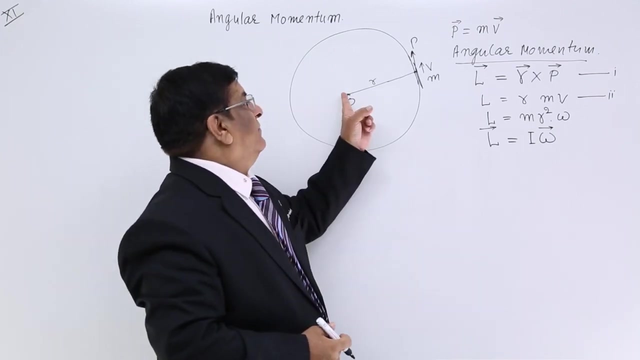 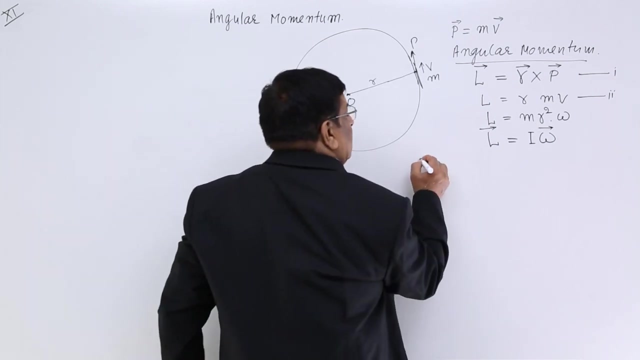 Direction along the axis, And that can also be seen from r and p. This is the direction of r, This is the direction of p And this is the direction of angular momentum. This is very important Because we have to learn so many things With this angular momentum. So angular momentum has got Is a vector quantity, It has got magnitude. 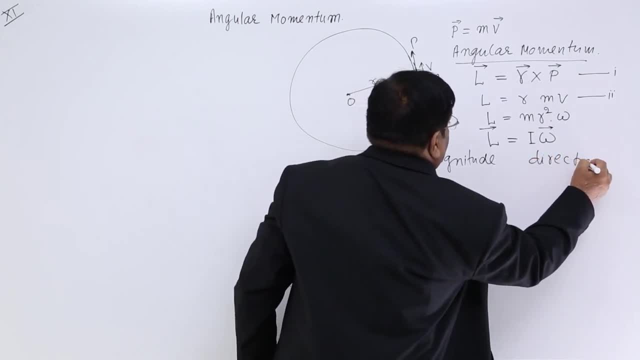 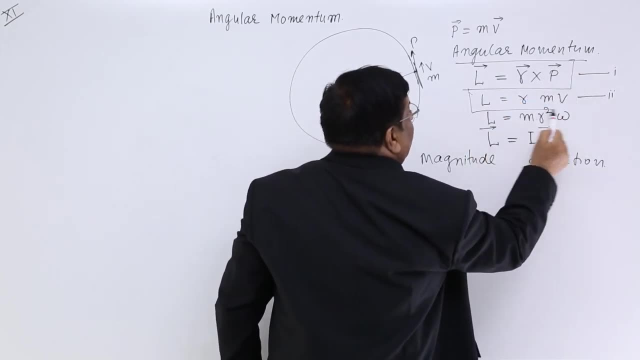 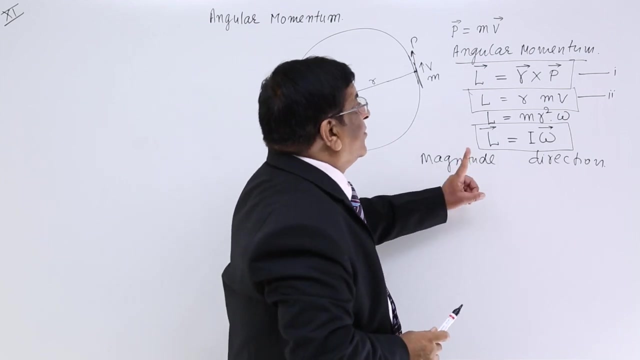 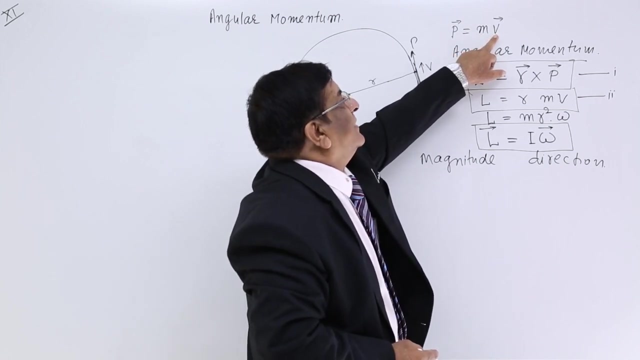 As well as In terms of linear momentum. This is our equation. This is our equation In terms of angular. This is our equation. Here, in the linear momentum, What do we have? Mass, That is inertia Multiplied by linear velocity. In rotational motion, Inertia is taken up by 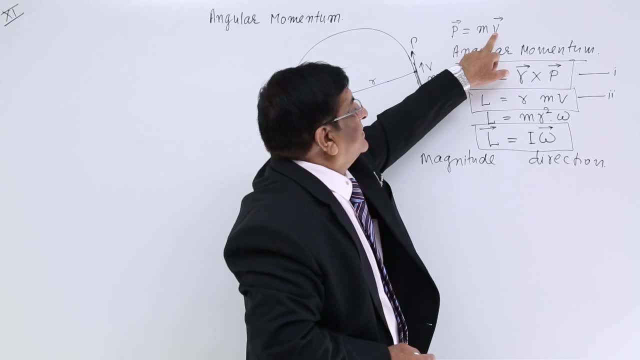 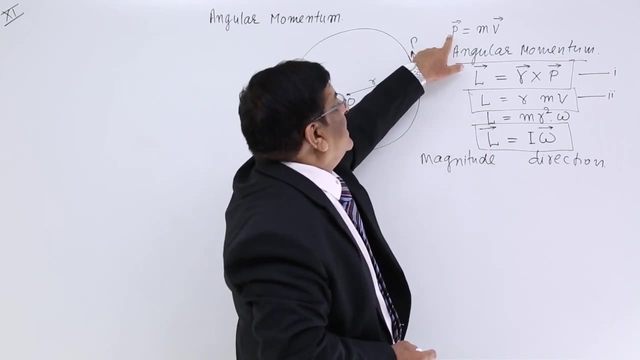 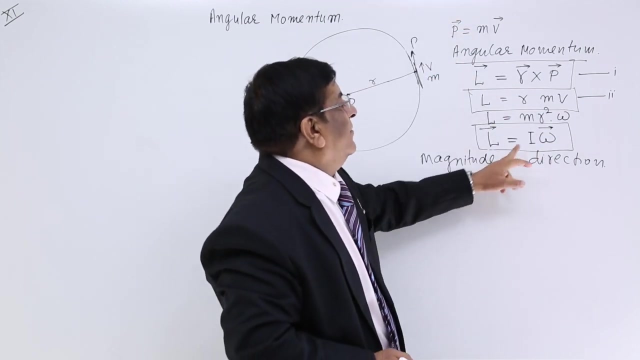 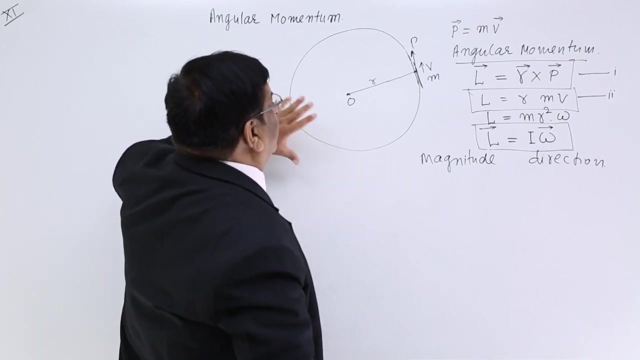 Moment of inertia. Inertia, Linear velocity, is taken up by angular velocity. So momentum, this is linear, This is angular. So momentum remains same. Only we have a conversion to linear, to angular. So this is angular momentum. Now we have the similar type of calculations, What we have for torque, If we take these two quantities, This is a cross product. So we are taking 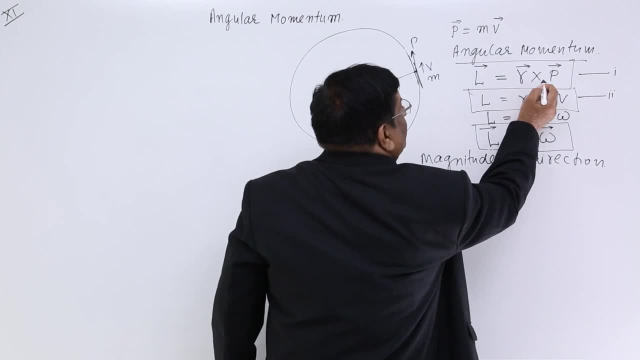 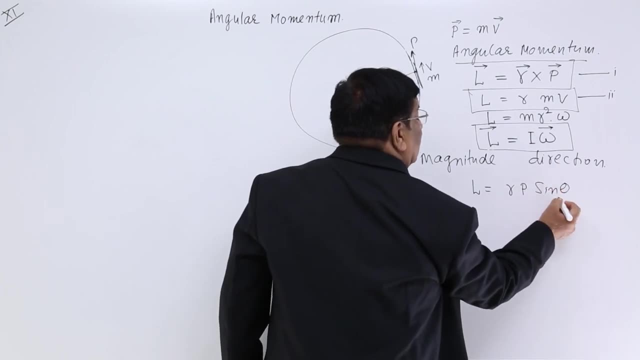 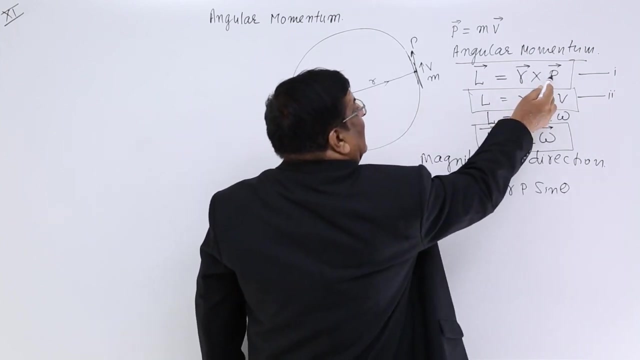 E, E, E. We are taking E, E, E product, and this tells us that L is equal to r, p sine theta. What is this theta? Theta is the angle between position vector r, position vector r and p. Here it is 90 degree. If it. 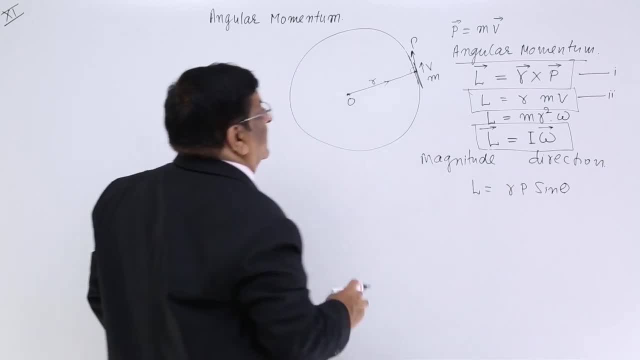 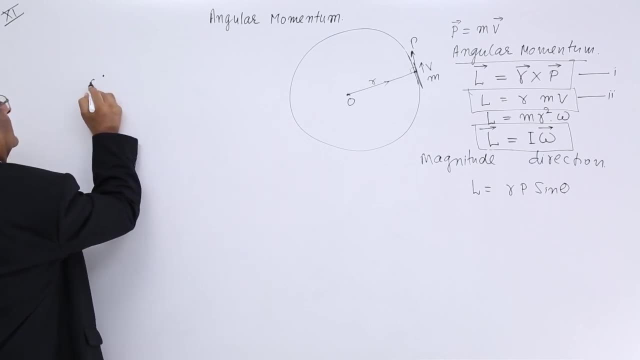 is 90, sine 90 is equal to 1.. Okay, if it is not 90, then see, we have two methods, The same way we have it there. This is a point of rotation o Here at the position r, there. 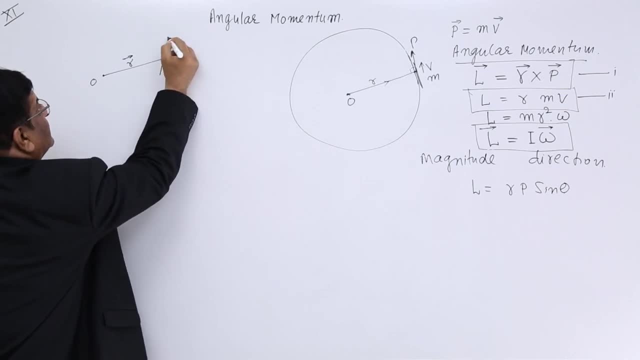 is a point p where we have this mass m moving in this direction, v. So what is this direction? This direction is direction of linear momentum. Okay, the angle between position vector and linear momentum vector is theta. Now you know, p can be divided into, p can be resolved into two components. One component: 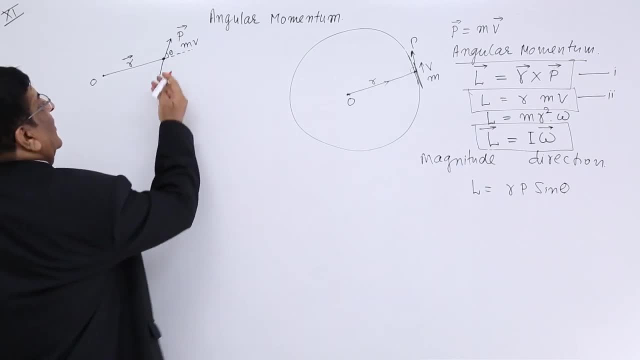 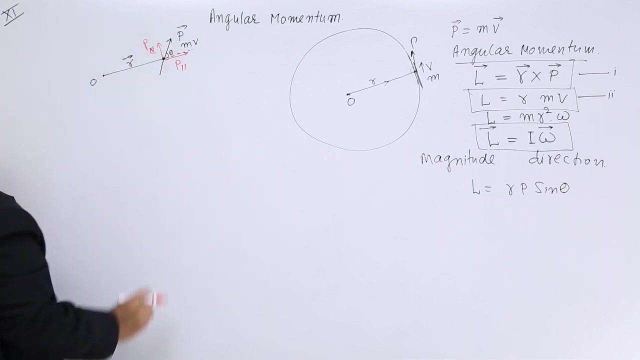 is parallel to the position vector, and we will call it this: p parallel, and here p perpendicular, p normal For rotational momentum. which component is parallel to the position vector? This is the component that is effective. Answer: this is effective because this makes the rotation. 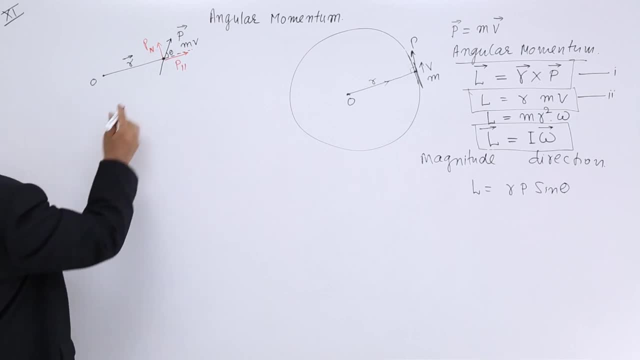 So p normal into r gives us angular momentum. L is equal to r multiplied by p normal. And how much is the magnitude of p normal? The magnitude of p normal? this magnitude is p cos theta And this magnitude is p sin theta. So when we are calculating the magnitude of l, it 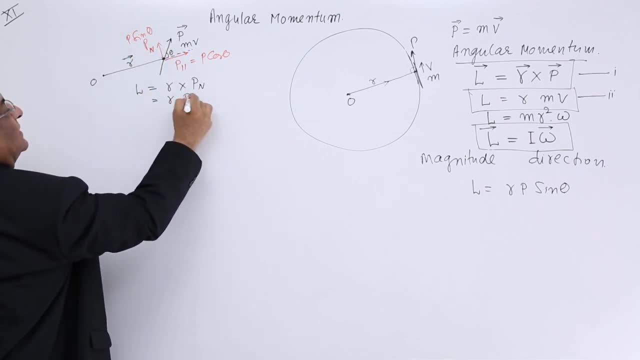 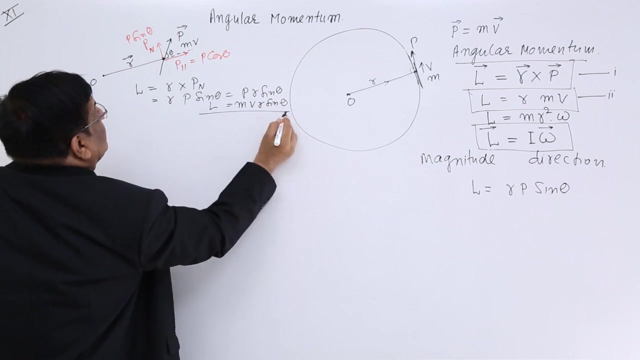 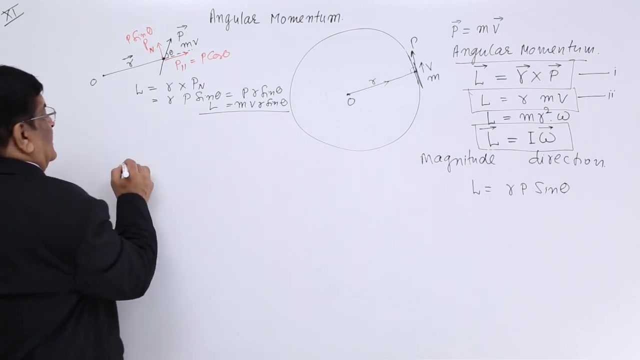 is r into this p sin theta. So this is p r sin theta, Or you can write it: mv r sin theta. Yes, Now we can see that what we have resolved is here. the momentum Now. again, this is: 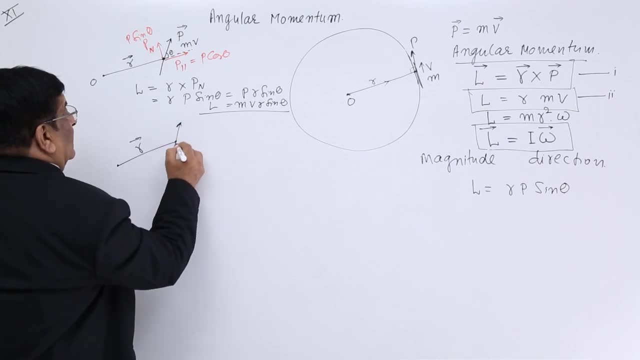 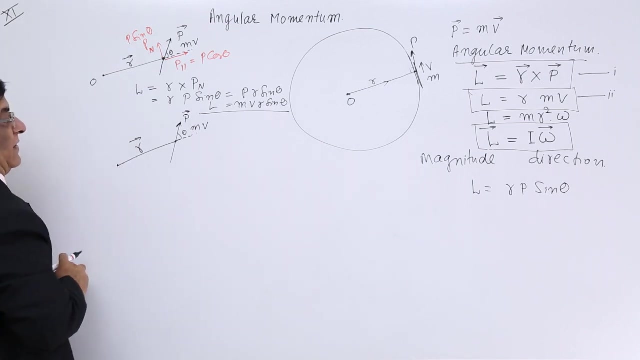 position, vector r, and here this has got mass m moving with velocity v, So that p is the direction of momentum. Okay, Okay, Okay, Okay, Okay, Okay, Okay is theta. Here we resolve P. Here, we don't want to resolve P, We will resolve R. So 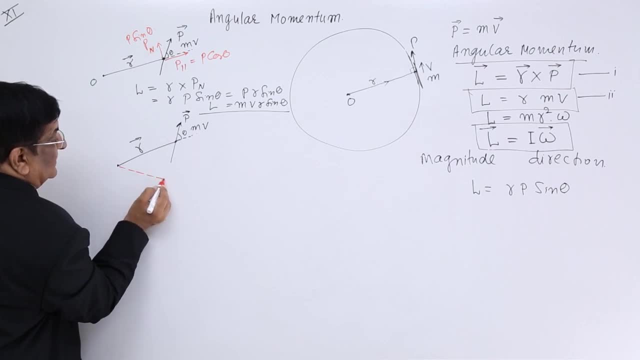 one resolved into two vectors. This is one vector which is perpendicular to the direction of velocity, direction of momentum. Other one is parallel. Here we complete the parallelogram. So this is one component, This is other component. This component we will name as vector R, which 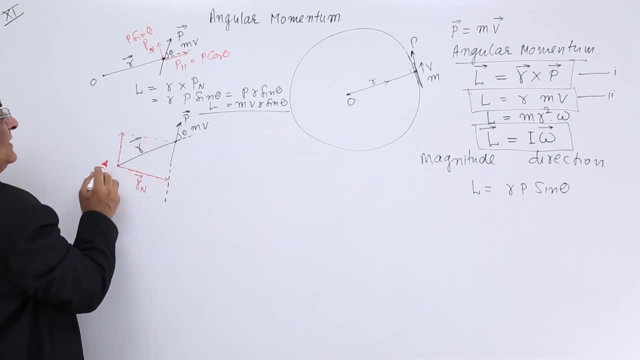 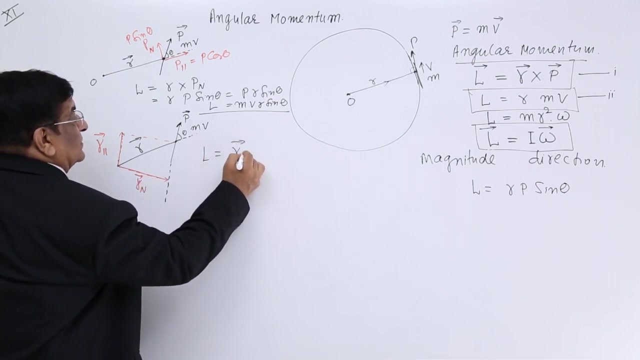 is normal to P. This is vector R, which is perpendicular to P. Now to get the rotational effect, which component is to be taken? We have to take the normal component. So angular moment of momentum L will be given by R, which is normal to be multiplied with P, And how much. 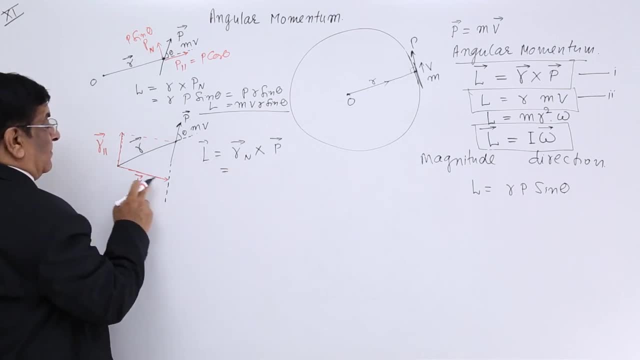 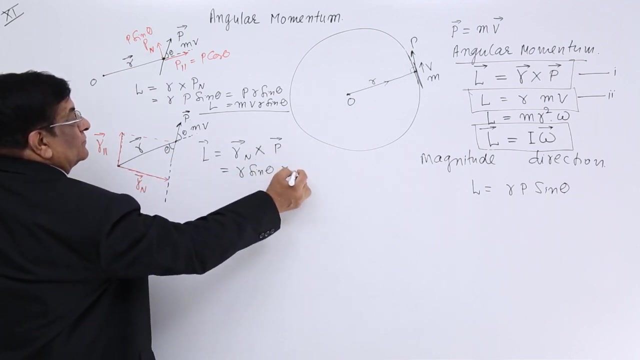 is R normal. R normal is equal to: this is theta, this is theta. this is base, this is perpendicular. So this is R R sine theta. This is P, So this is P. So any acceleration is история. Another one will be those 그 немного Mv R sine theta. 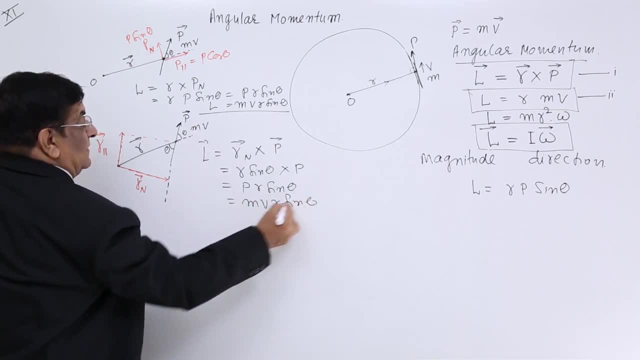 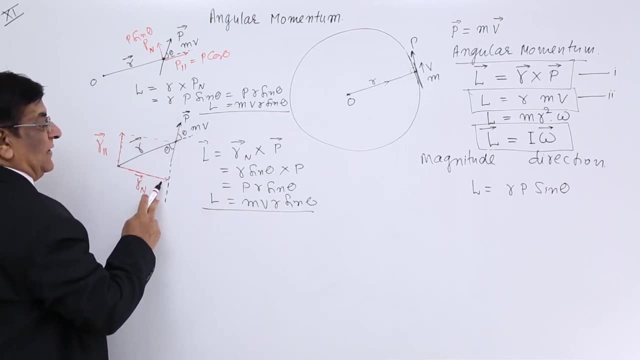 or Mv R sine theta, ie when we have resolved R. So whether we resolve R perpendicular to P, We get this result Here. we resolve P perpendicular to R, we get is 지긊 to the Mv R sine theta. that is when we have resolved R. Everyone. is familiar with these associations, right, So every ratio becomes after this: trouve: If I dissolve R perpendicular to P, we get did this result Here. we resolve P perpendicular to R, we get this result Again in the case of R and P given to us in the form of Cartesian. 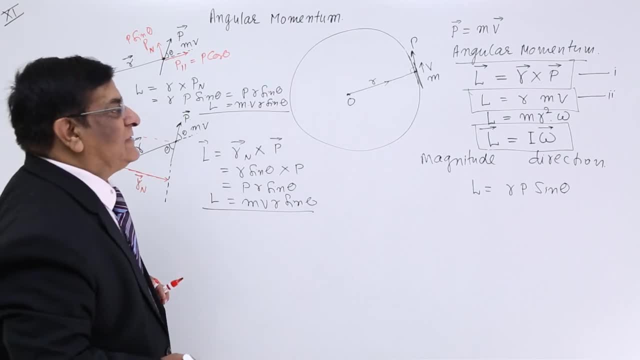 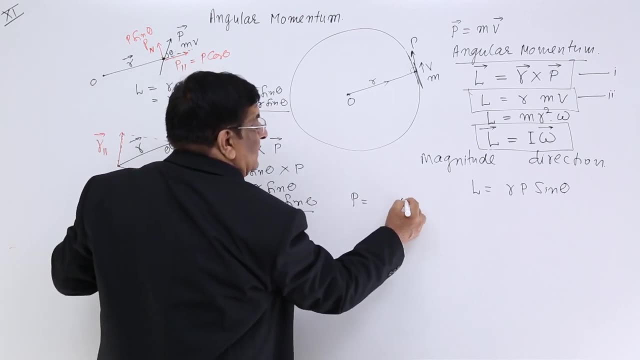 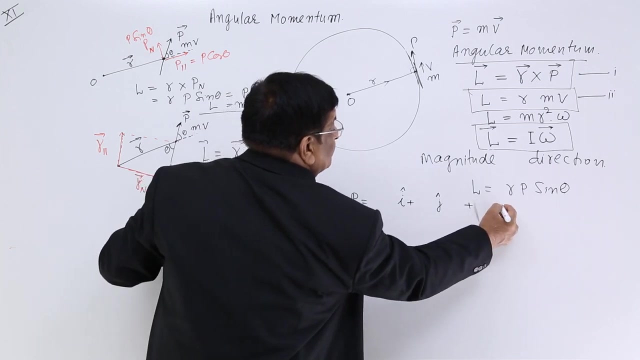 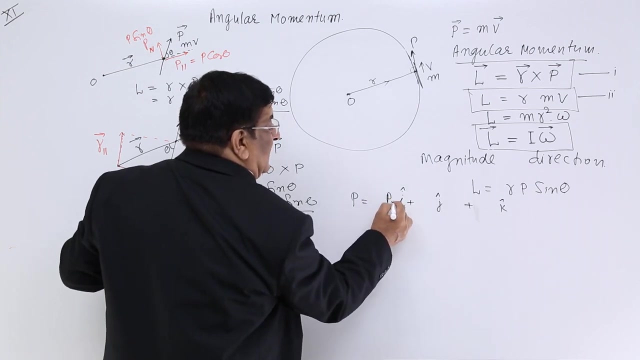 questions. let me recall, Let's take a look at the second set. Look at this one. If you, You will have the same formula here. like momentum, P is given to us i, j, k and they have certain multiplicant giving the magnitude, like Px, Py and Pz. 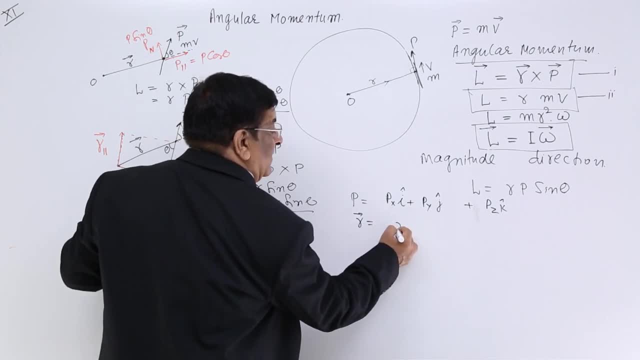 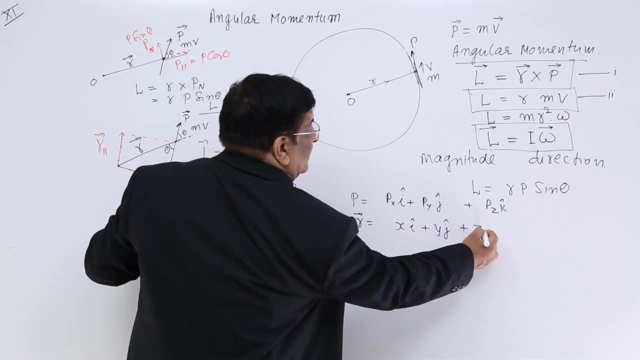 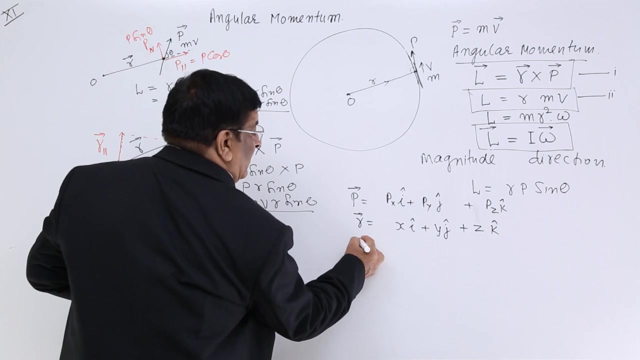 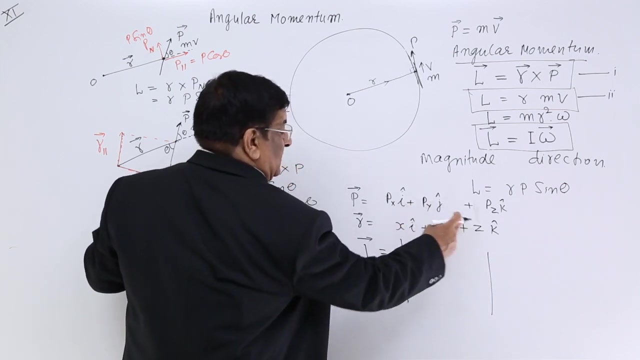 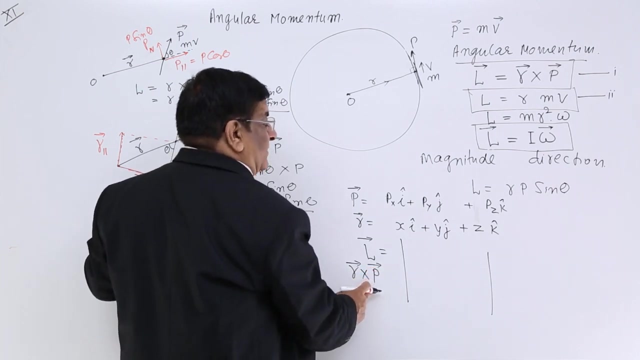 The position vector r is given by x in i direction, y in j direction and z in k direction, Then how much will be the angular momentum? The angular momentum will be cross product of the two, that is, r cross P. And how do we do the cross product? 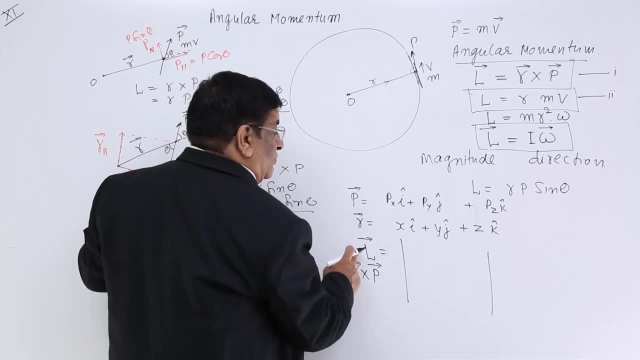 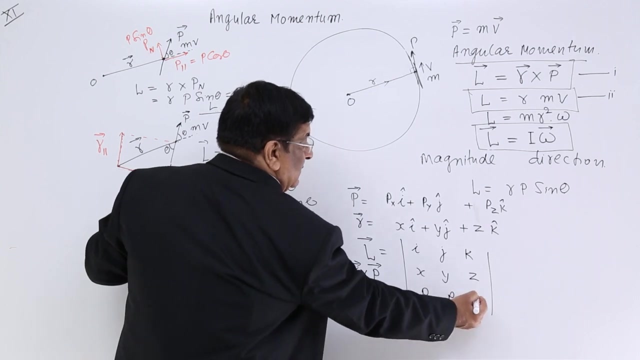 r is to be placed first, So doing the cross product. we will get the cross product in terms of i, j, k, First r components, r magnitudes x, y, z, Then P magnitudes of all three directions, Px, Py, Pz. 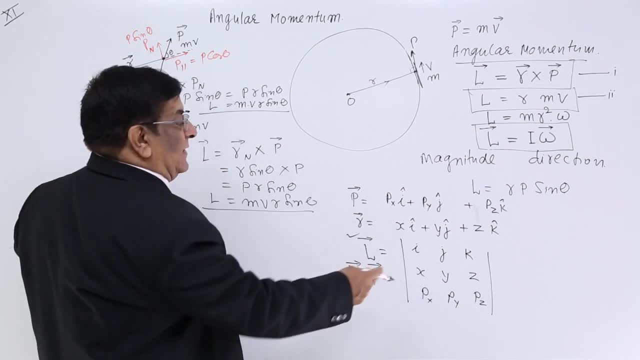 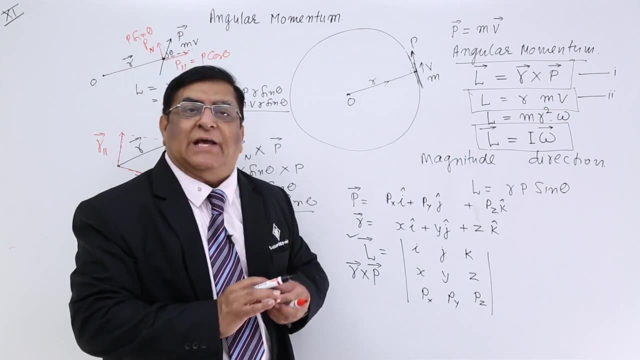 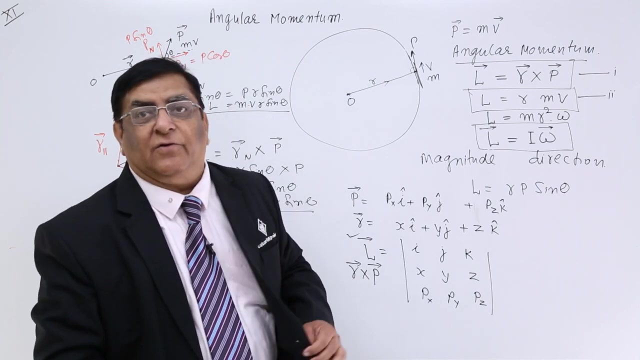 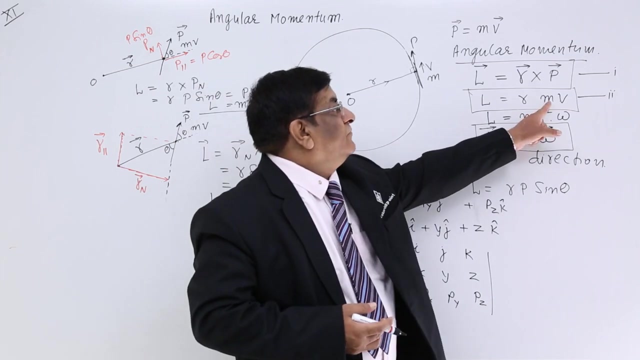 And here get the angular momentum when vectors are given to us in Cartesian coordinate system. So this is how angular momentum is calculated. So next, what should be the unit of angular momentum? The unit of angular momentum we can create by this formula: MVR, MVR, MV is 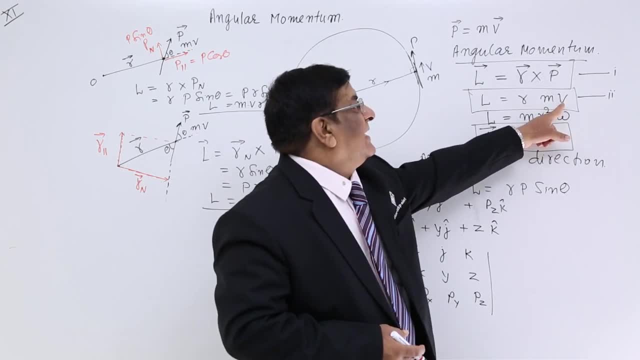 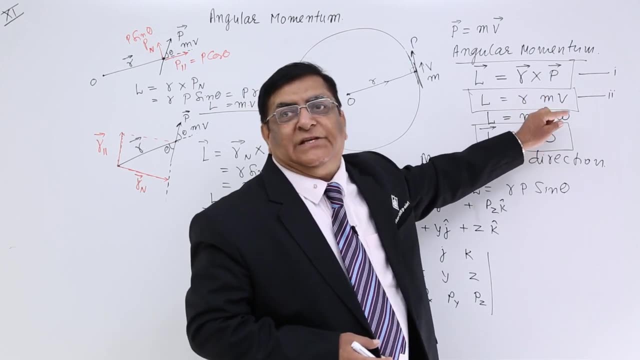 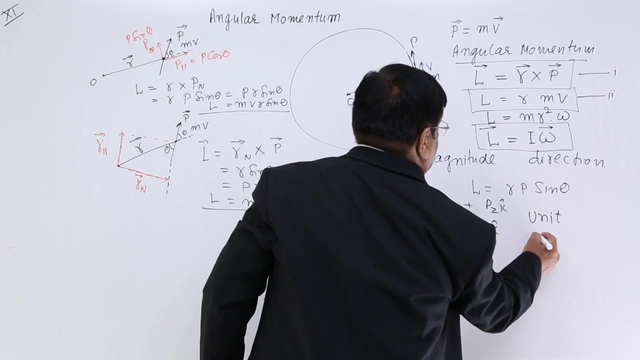 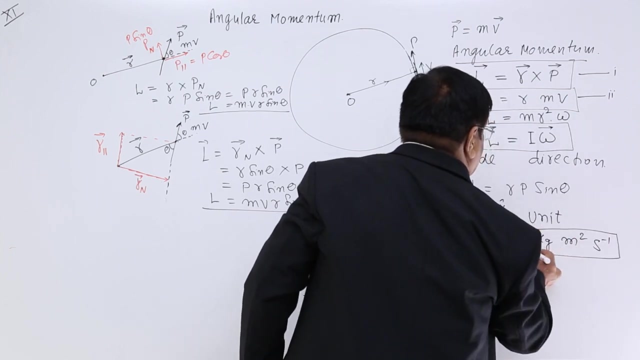 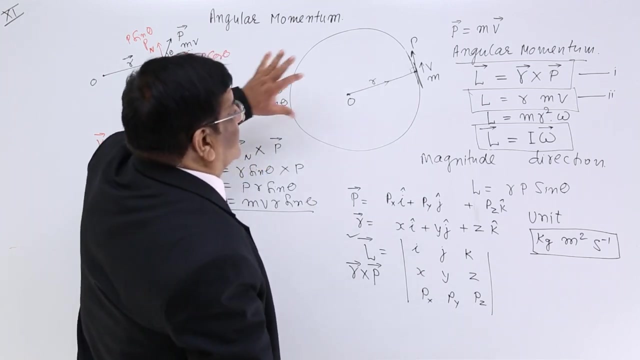 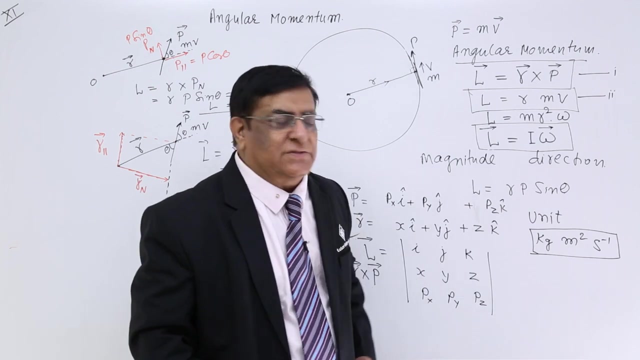 what Kilogram meter per second, and this R is again meter. Kilogram meter square per second. Unit: kg meter square per second. This is one unit. We can also connect it with other units. We will come to that. Okay, So this is how we can create this. With this, you can also find out its dimensions. 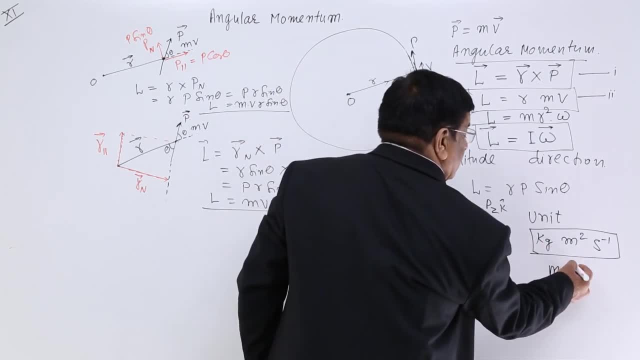 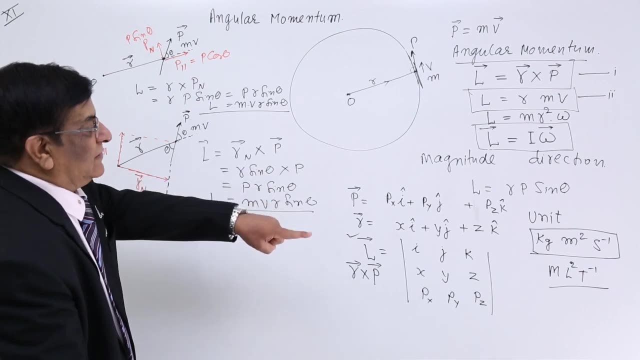 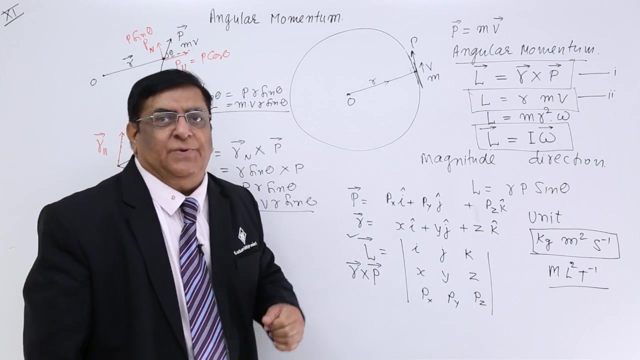 The dimensions. this is mass L2 t minus 1.. So this is- you can find unit dimensions, formula, calculations. and this is angular momentum. It is a vector quantity, So it must be having a direction that we have discussed. 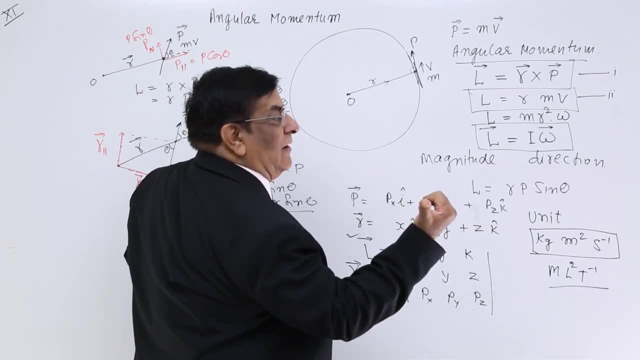 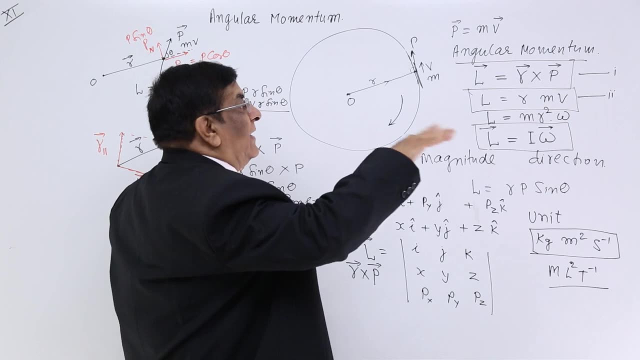 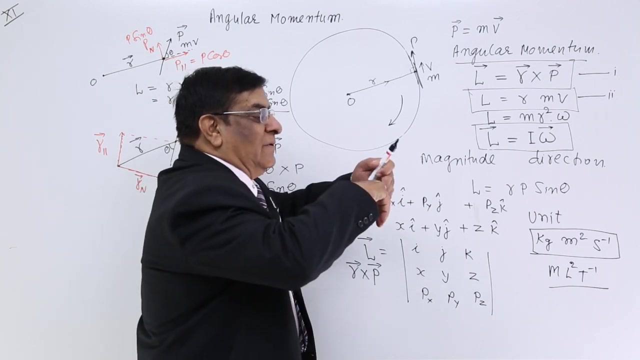 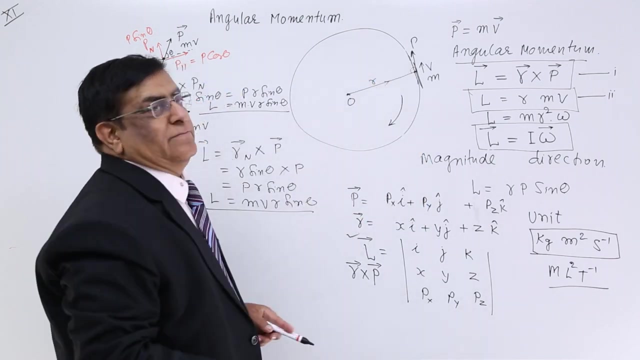 Okay, This is R, this is P, this is L. But if you make the rotation this way, then what will happen? R and rotation downward. So I have to put it this way: This is R, this is velocity, That is direction of MV down. So now it is inside, angular momentum inside. Okay, Now. 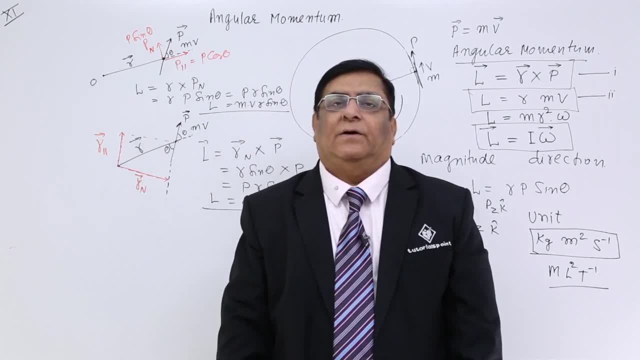 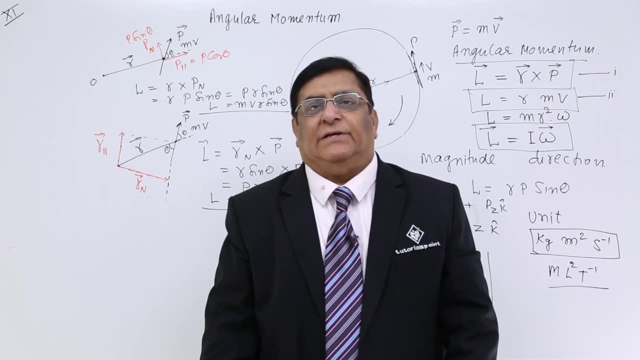 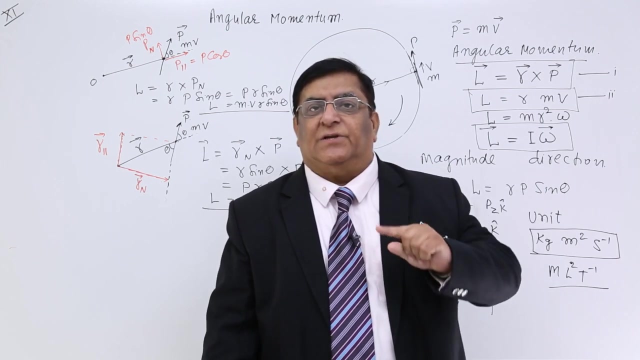 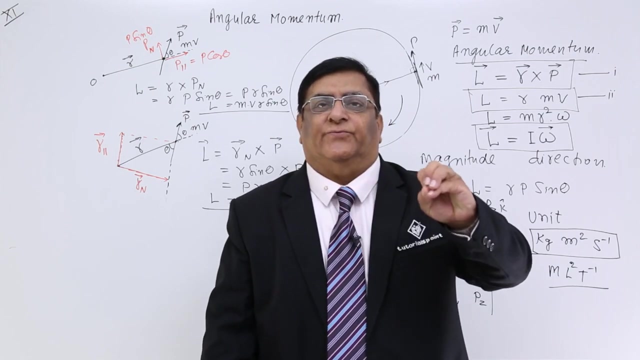 why do we give so much Stress on angular momentum? Because angular momentum is the quantity which is conserved If no external force in rotational motion. who is doing the work of force? Answer: it is torque which is doing the duty of force.